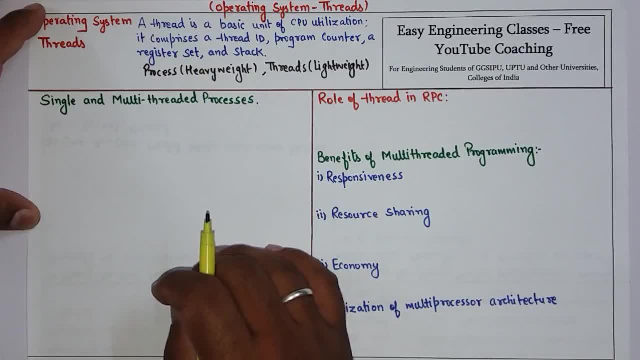 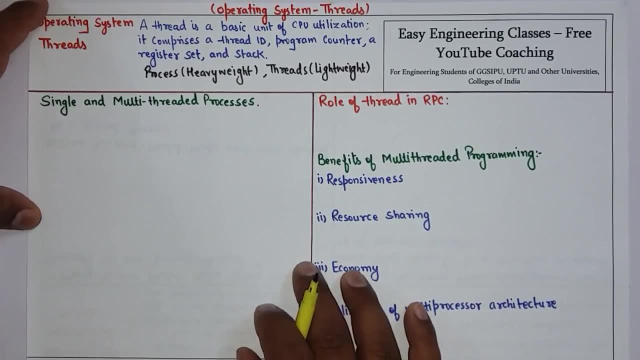 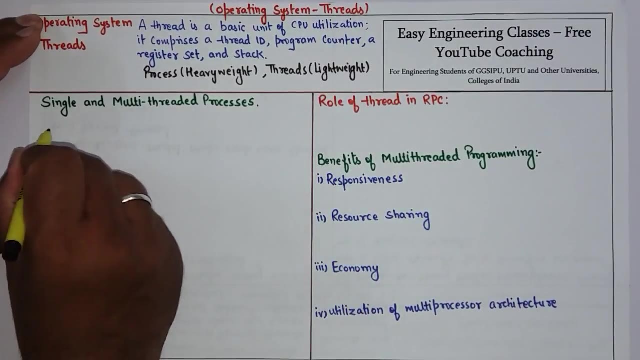 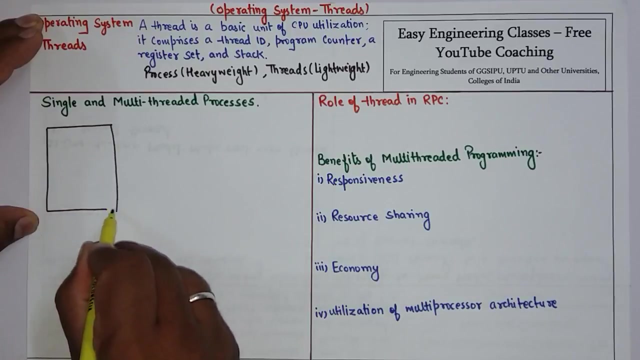 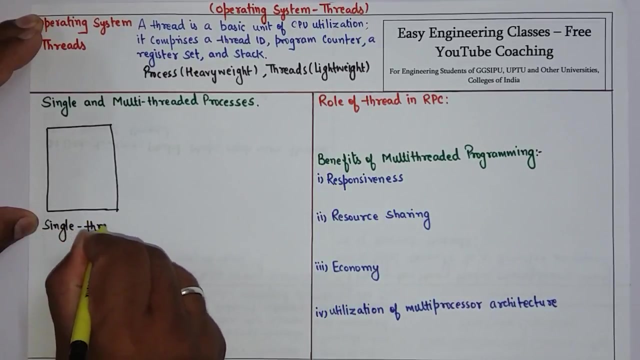 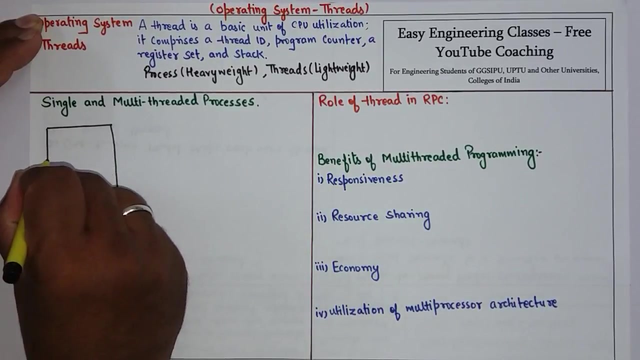 threads of control, then it is called as multi-threaded process, And that multi-threaded process can be used to perform multiple tasks at a time, So we can show those with the help of diagram. This is the single threaded process. In this we have some of the of the properties. 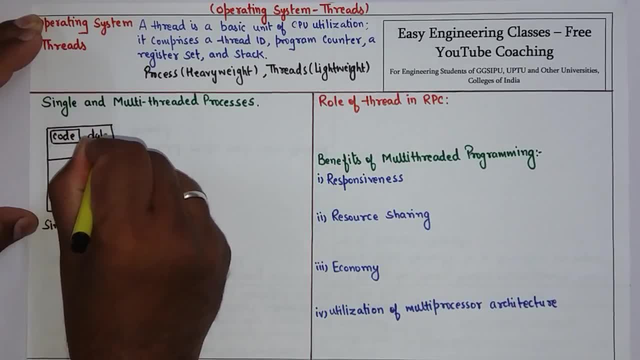 of process, like the code of the process data, than we have stack registers and lots, many other things. simple stumble, mother you can login after related to this software. Those are various names. they are from inside a data, many things that are present in any process. 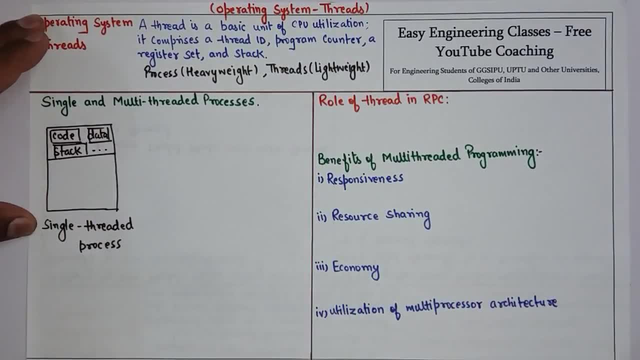 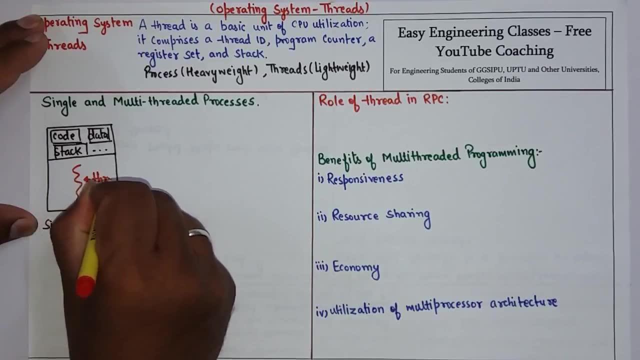 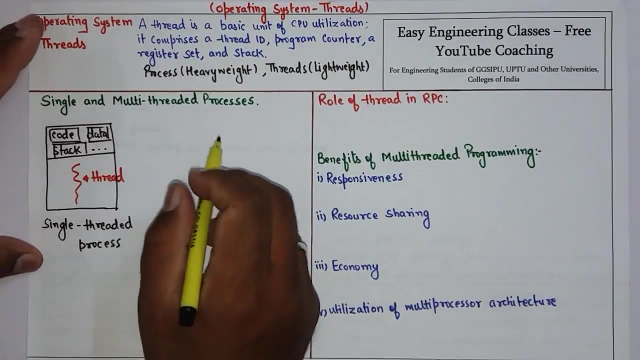 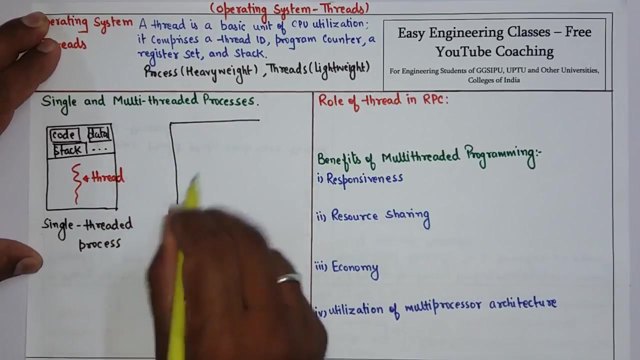 And if this process is handled by a single thread, then it is single thread of process. Suppose this is the thread. since there is only one thread, it is a single threaded process. But if, for example, this single threaded process is converted into a multi threaded process, 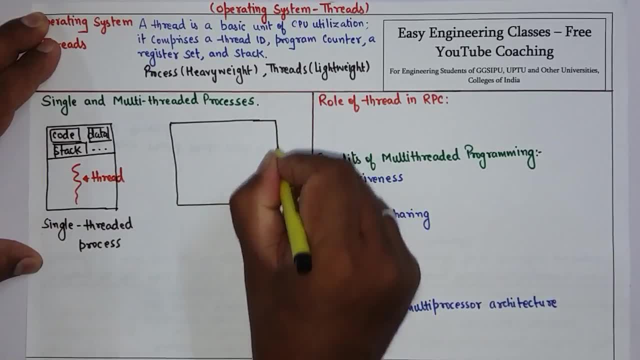 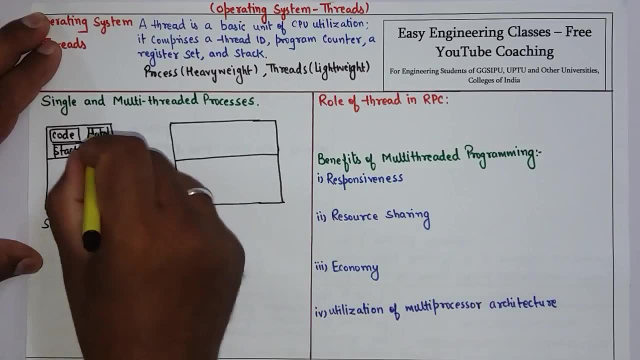 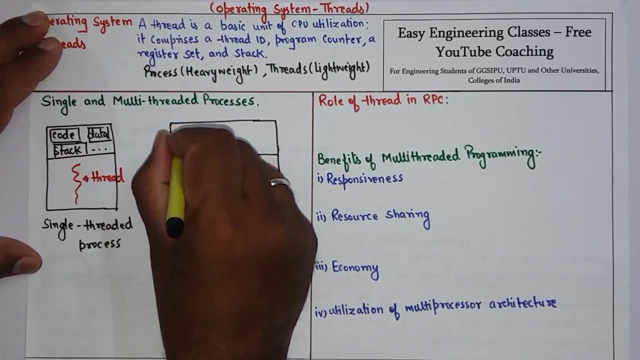 that means the process. this process is now controlled by multiple threads. In that case, the resources are also shared by all the threads. So for each of the threads, depending on the type of resources it needs porta, these resources are shared. So, for example, if one thread is requiring only the code along with register and stack, 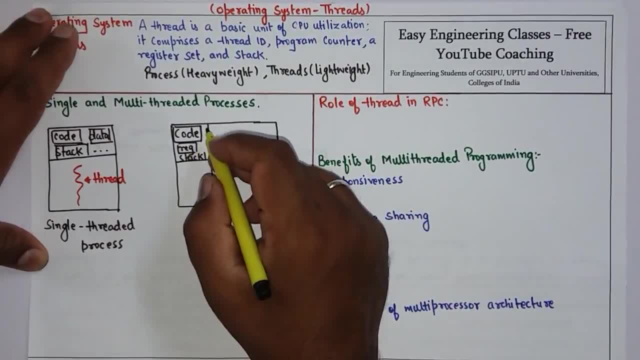 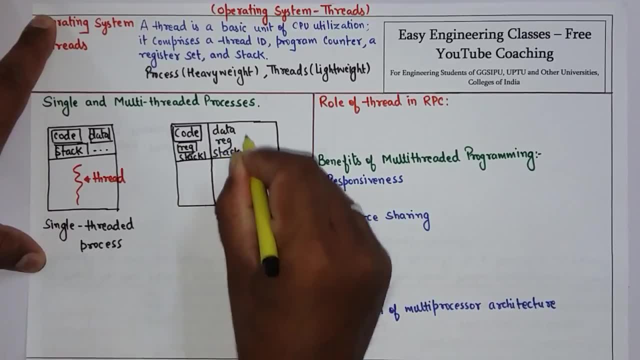 then this thread will get access to these resources. Similarly, if another thread is requiring data register and stack, then this thread will get access to these. In this you can see that the register and stack resources are shared Again. also, if one of the thread require files register only, then these resources are also. 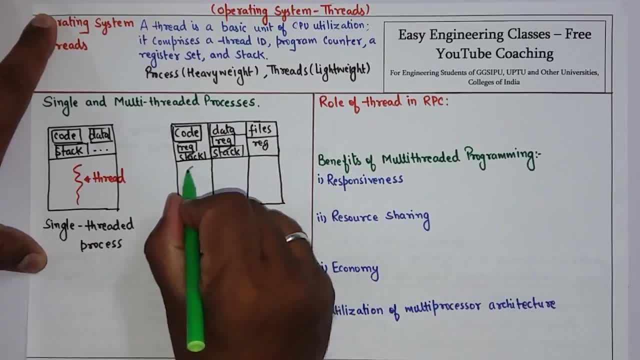 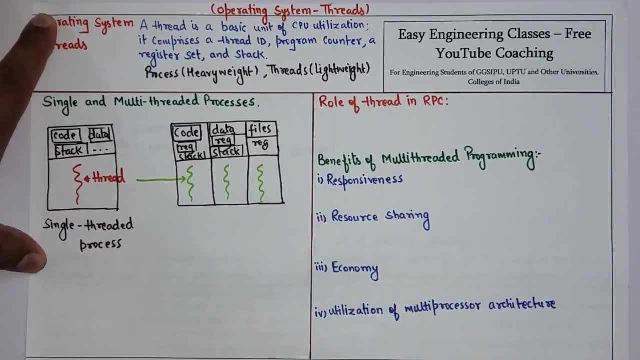 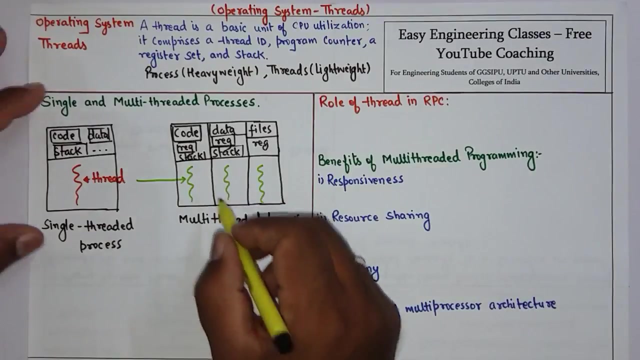 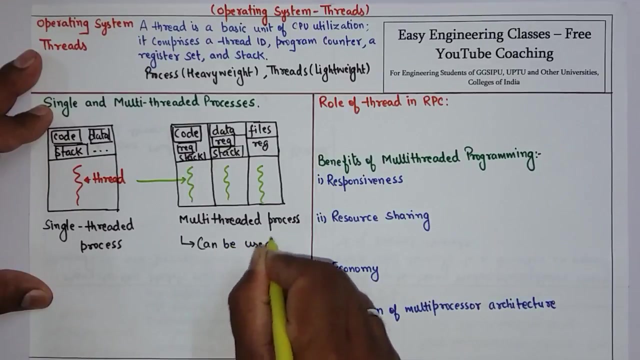 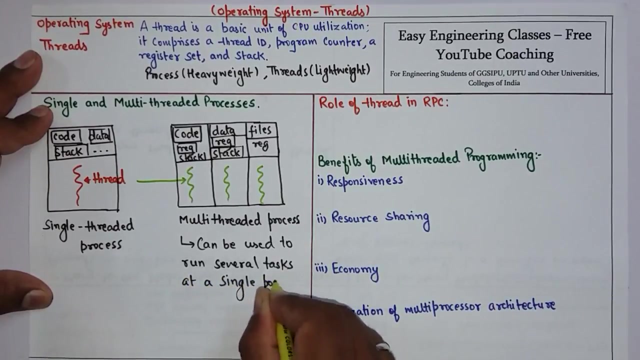 shared. So in this, for each section, we have different thread. So this is your multiple or the multi-threaded process. Now, what is the benefit of this multiple or the multi-threaded process is it can be used to run. can be used to run several tasks at a single point of time. 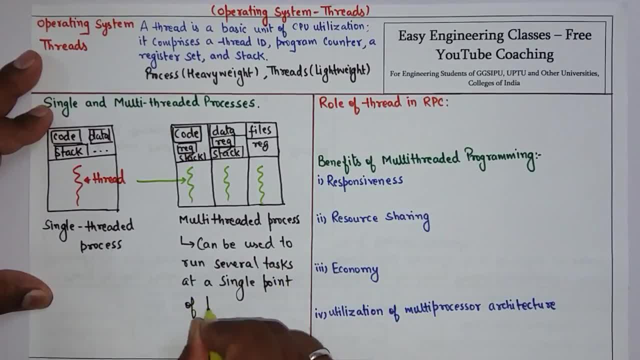 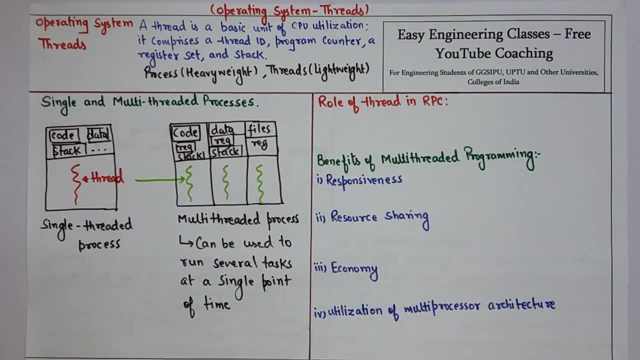 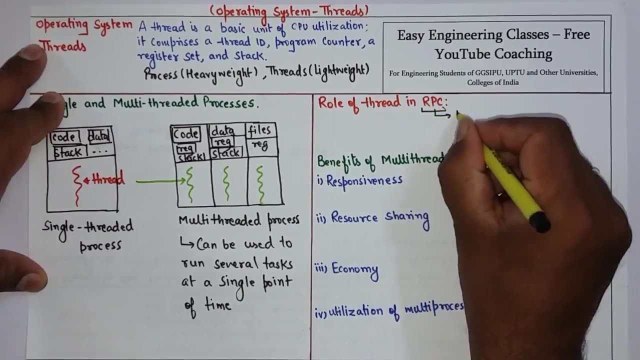 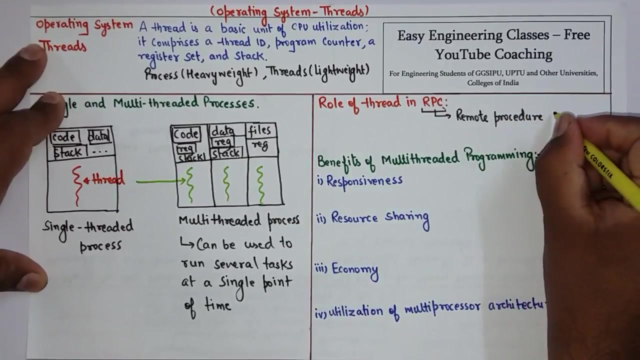 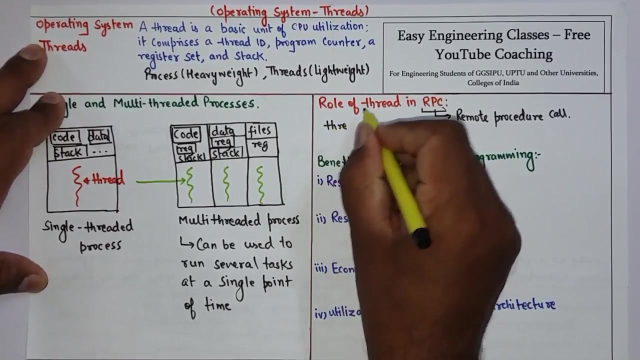 That is your multi-threaded process. Thank you. Now threads also play a vital role in the RPC. that is remote procedural call. This is your remote procedure call. Remote procedure call is used to call a function of some another program. Threads can also be used for this, because threads can be used for inter process communication. 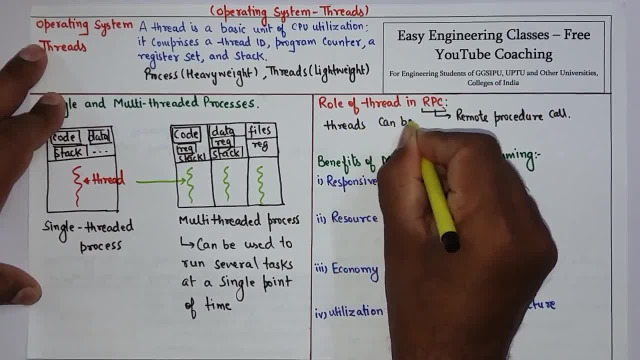 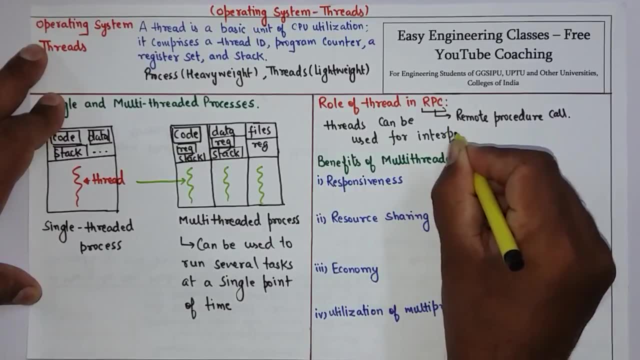 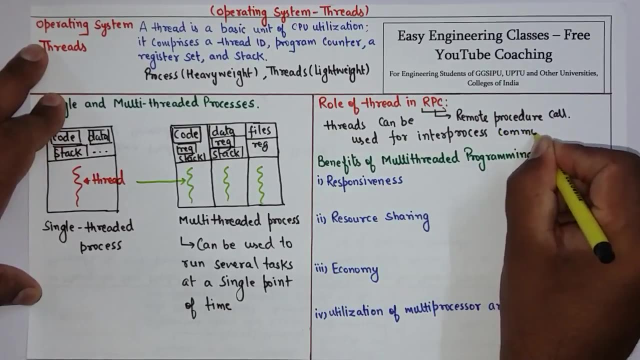 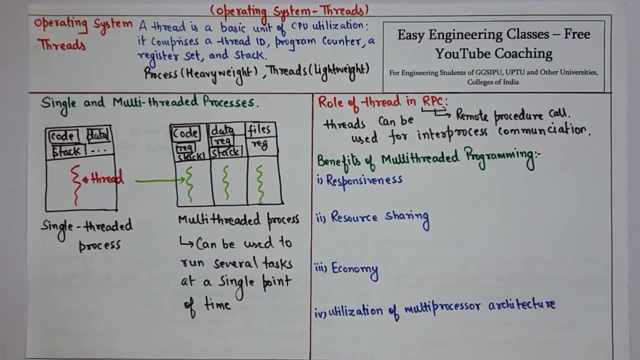 So threads can be used for inter process communication. So threads can be used for inter process communication. So threads can be used for inter process communication. That is how threads play a important role in RPC, with the help of inter process communication. Now we will see some of the benefits of the multi-threaded programming. 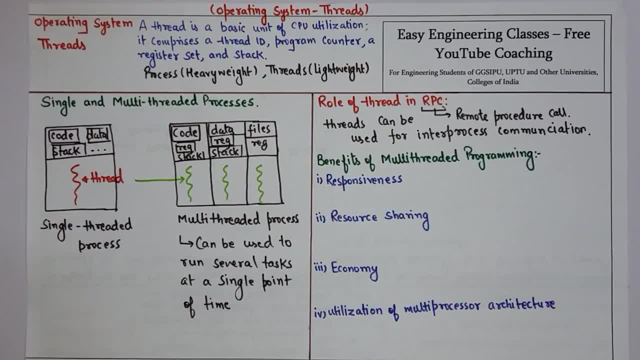 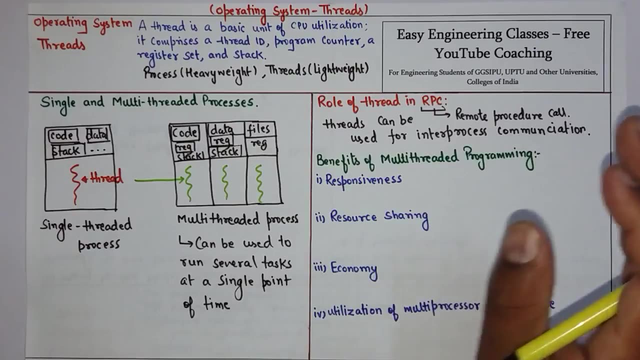 The first benefit is responsiveness. Responsiveness, Since the multi-threading is an interactive application and it allows a program to continue running even if a part of it is blocked, So that increases the responsiveness to the user. For example, suppose this particular section is not responding. 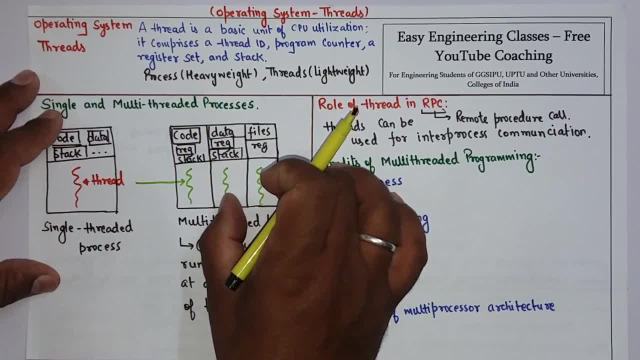 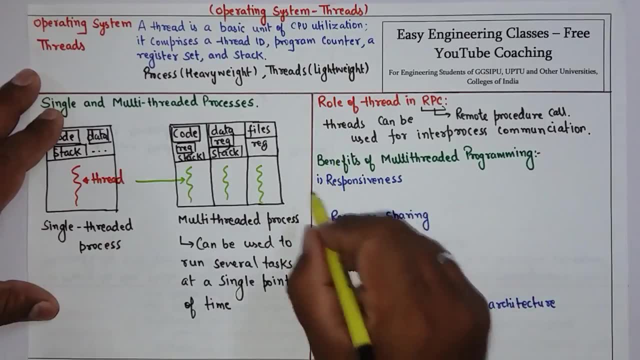 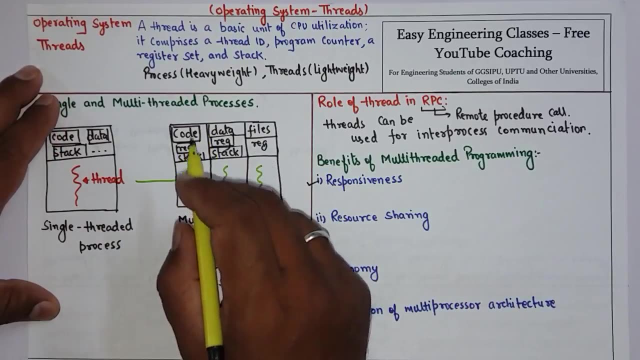 Then instead of entire process not responding, these two sections can respond to the user. that give more responsiveness to the user. So that is your responsiveness. Then we have resource sharing. As we have seen here, threads share the memory and the resources of the process. 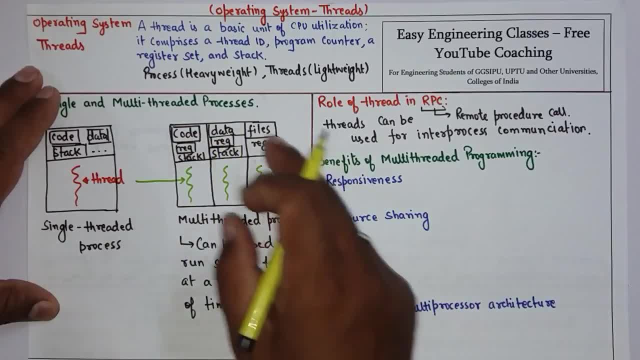 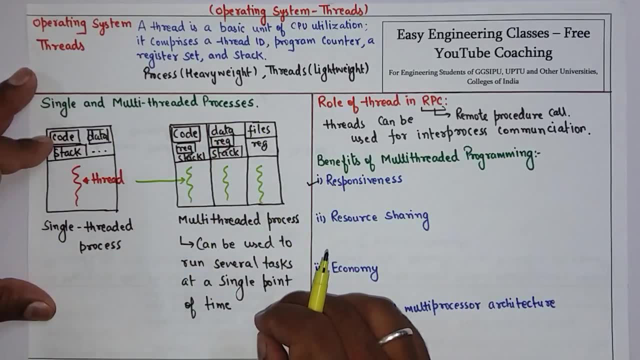 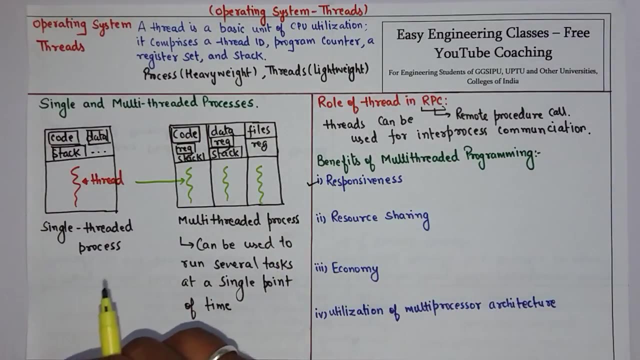 So, whatever memory the process has, that memory is shared by the user, by the thread, and the resources are also shared by the thread. Now, the benefit of sharing code and data is that it allows an application to have several different threads of activity within the same address space. 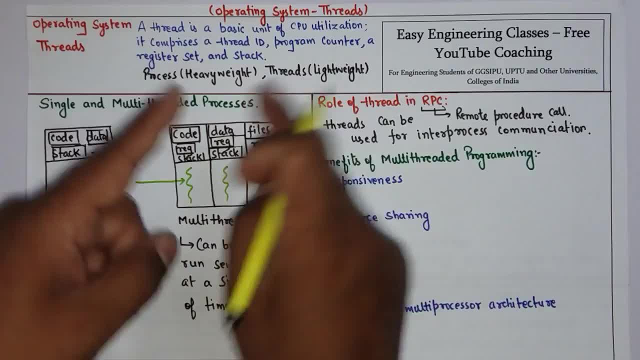 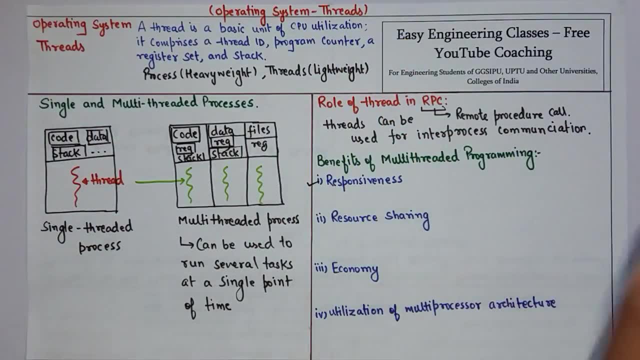 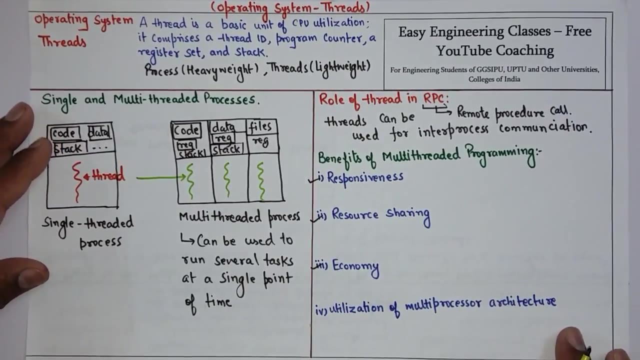 So that is what we have seen here. Three different threads are running in the same address space. So by running in the same address space, the inter-process or inter-thread communication is also cheap. Then the third benefit is the economy. Economy means allocating memory and resources for a process. creation is costly. 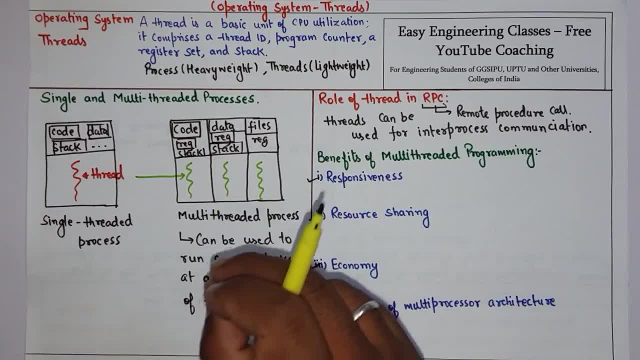 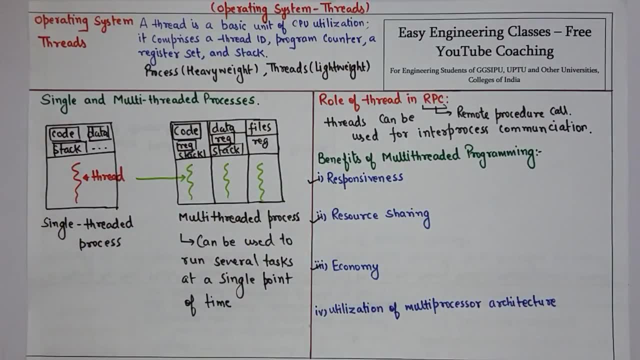 Now, since threads are created by the user, The process is created by the user, The process is created by the user, The process is created by a process and share its resources also, So it is most economical. Then, instead of creating a process for every request, we can create a thread for that particular. 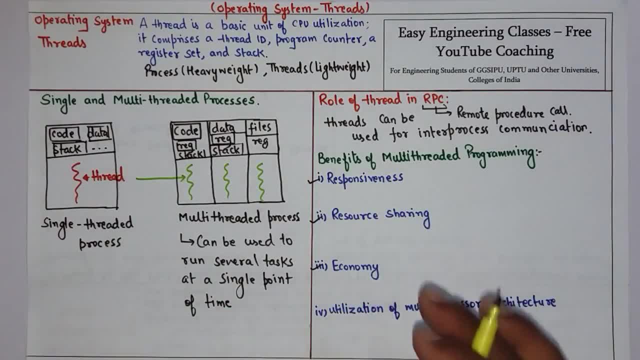 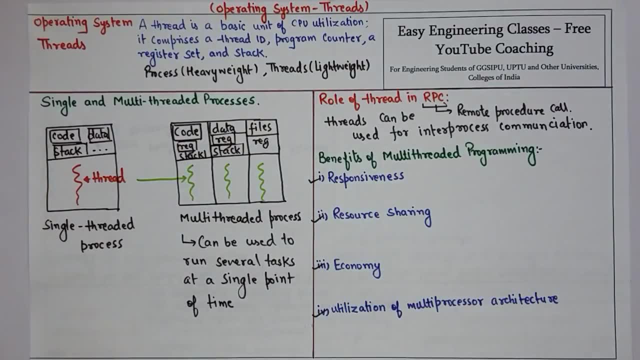 request. So that gives benefit to the economical point of view to the system. Then the final benefit is utilization of multi-processor architecture. The benefit of multi-threading can be greatly increased in the multi-processor architecture in a way that threads may run parallelly on different processors. 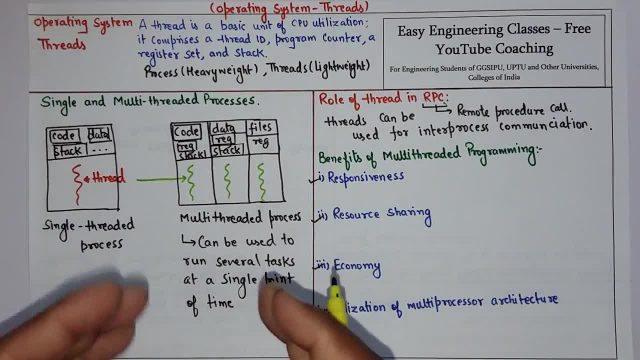 So if we have different different processors in multi-processing system, then the threads can be made to run concurrently on different processors. So that increases the concurrency Because a single thread process can only run on one CPU, no matter how many threads are available or how many processes are available. 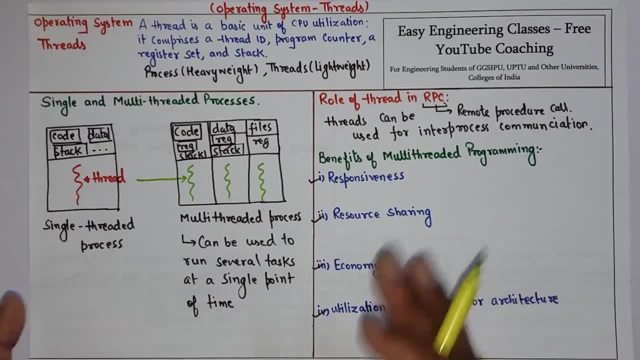 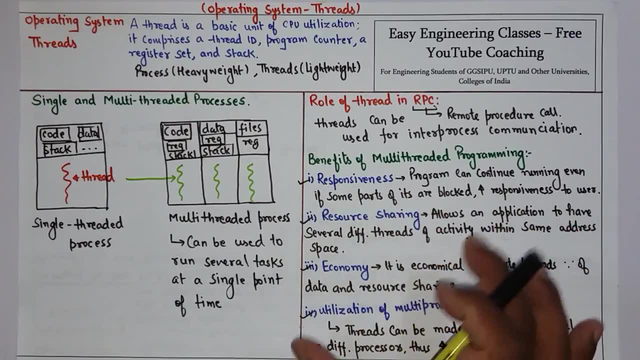 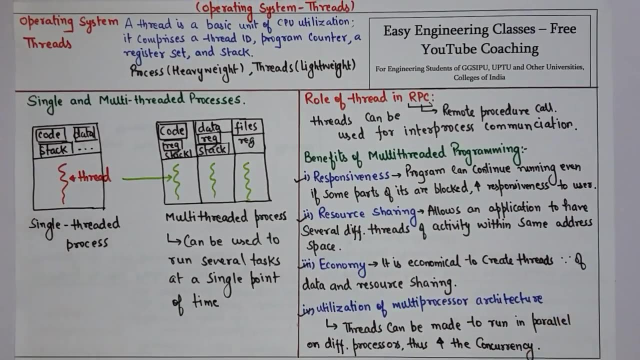 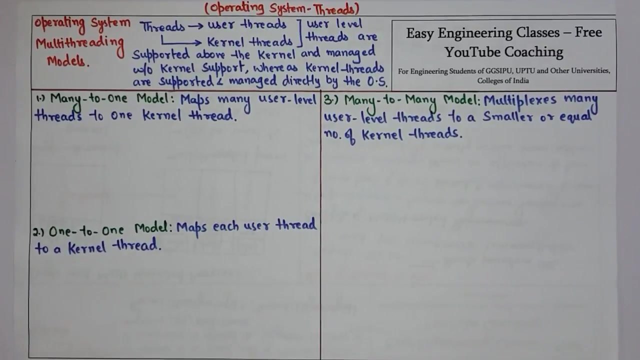 So we are actually utilizing the multi-processor architecture by using multi-threading. So these are the benefits. I have written important points of these benefits of the multi-threaded programming. You can note it down from here. Now let's move to the multi-threading models. 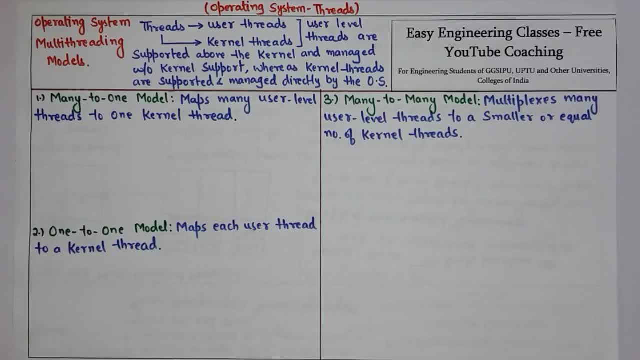 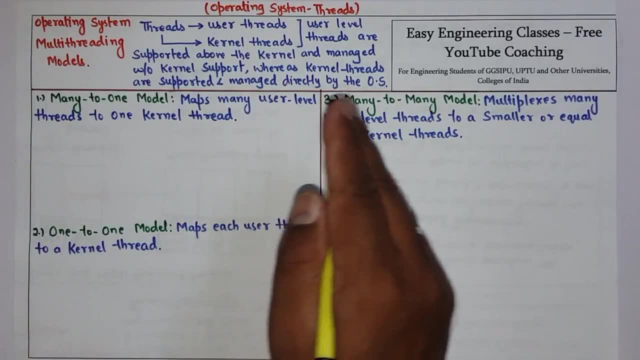 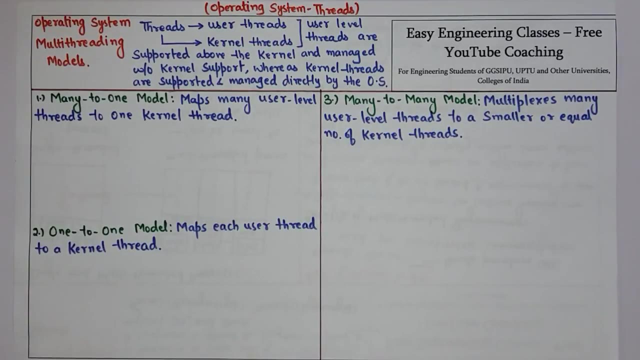 Threads can be of two types: user thread and kernel thread. User level threads are supported above the kernel And managed without kernel support, whereas the kernel threads are supported and managed directly by the OS. There are different models for the mapping of a user level thread to the multi-level. 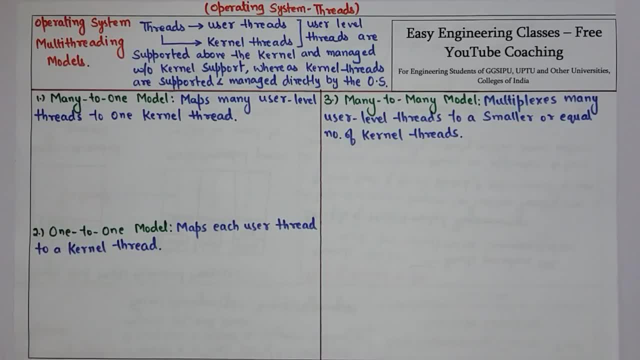 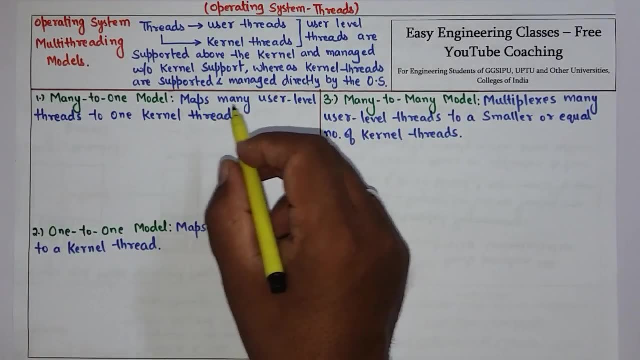 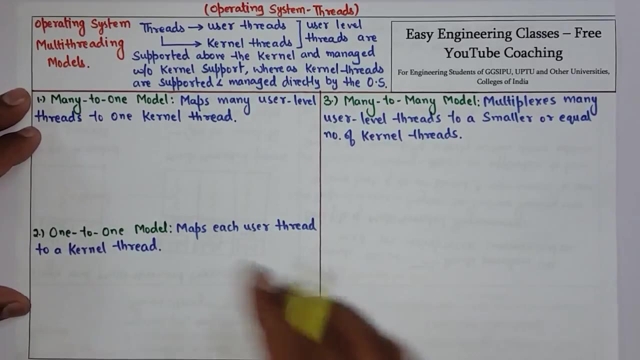 thread. So we are going to discuss each of this level, each of this model. The first model is the many to one. In this the mapping is done between many user level threads to one kernel level thread. So it is Shown like this: 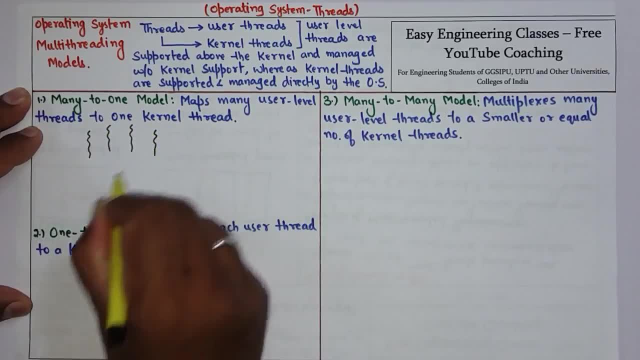 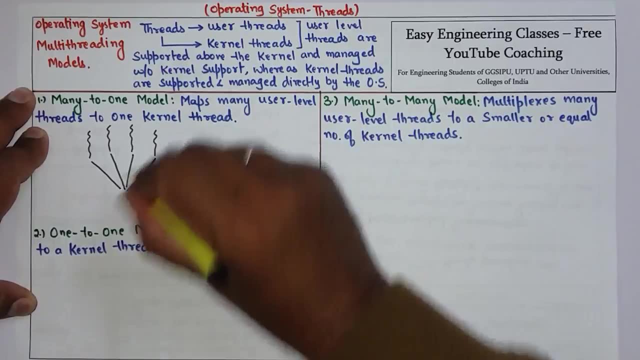 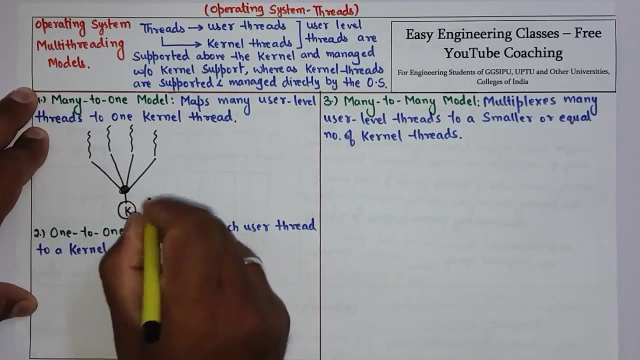 So we have many user level threads here And these user level threads are mapped to a single kernel thread. So this is the kernel thread And these are user Thread Threads. So this is many user level, many user threads and one kernel thread. 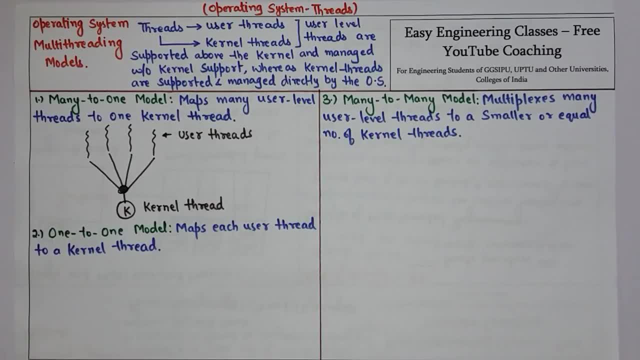 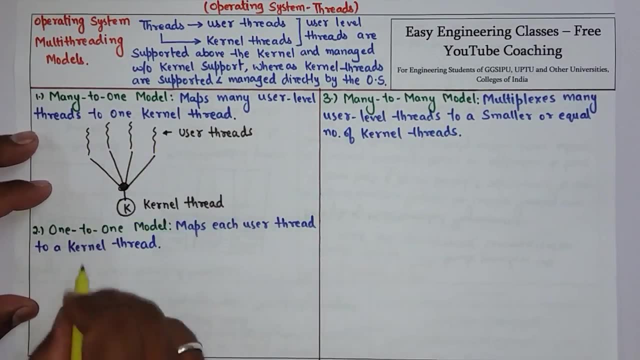 Then we have one to one model. One to one model says the mapping is done between each user thread and kernel thread. So if we have these four user threads, then for each of these four threads we will have one kernel thread. That is the one. 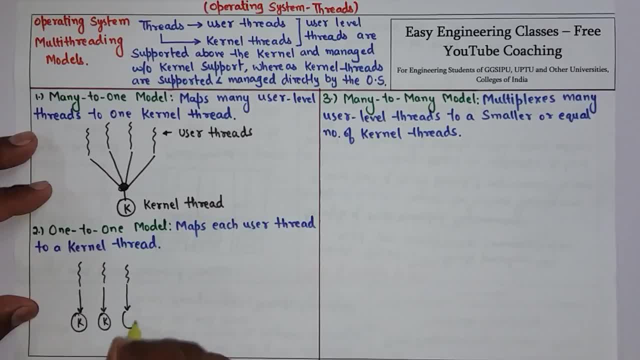 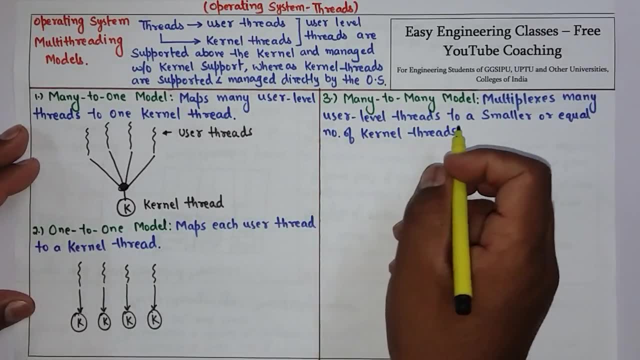 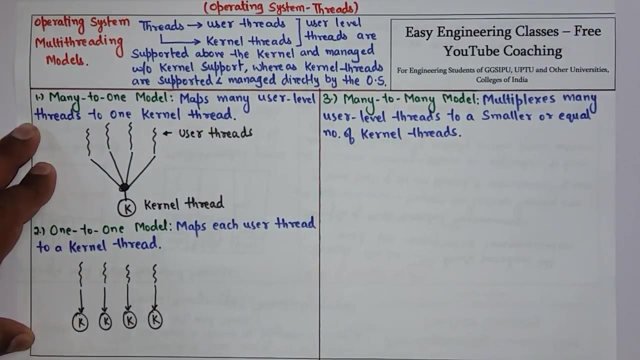 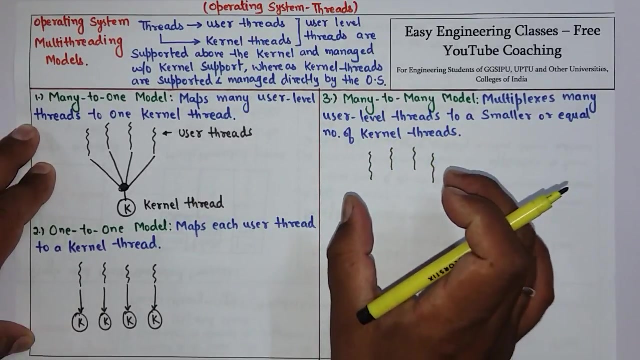 Thread Thread Thread Thread Thread. Then we have the many to many model. It multiplies many user level threads to smaller or equal number of kernel threads. So in this, if we can, we have this four user threads, then we can have either four or less. 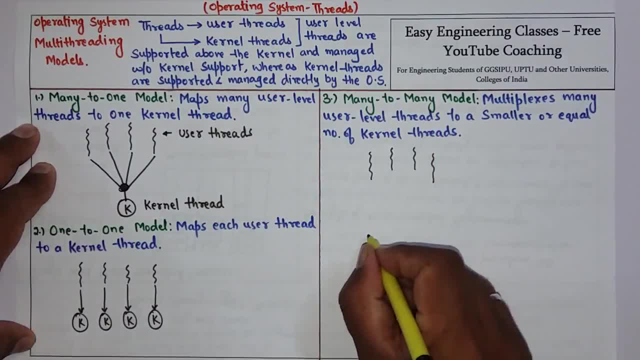 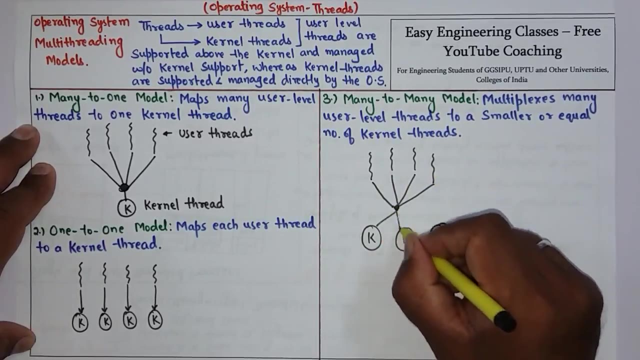 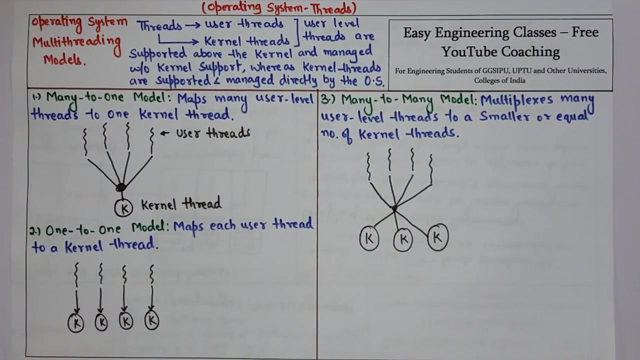 than four kernel threads. So, for example, we have three kernel threads here. then there is a multiplexing kind of thing like this, in which these four user level threads are managed by this three kernel level threads. that is your many-to-many model. so this is about the threading concept. 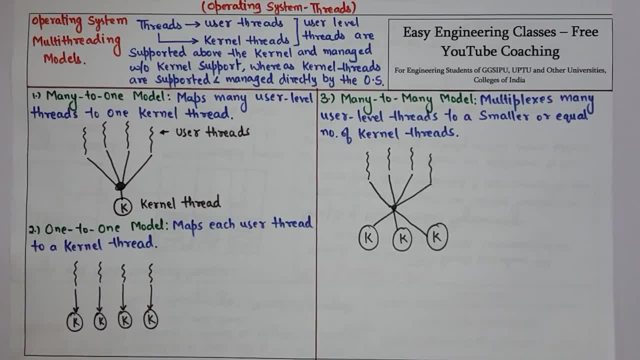 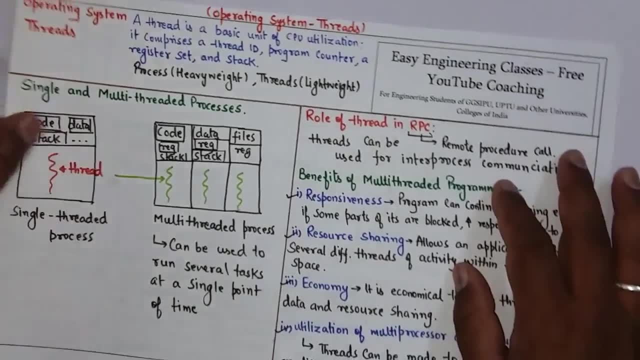 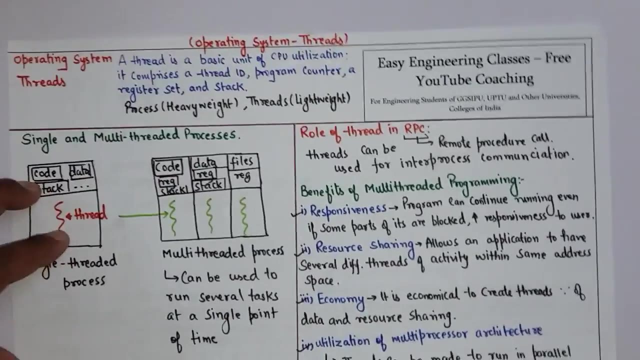 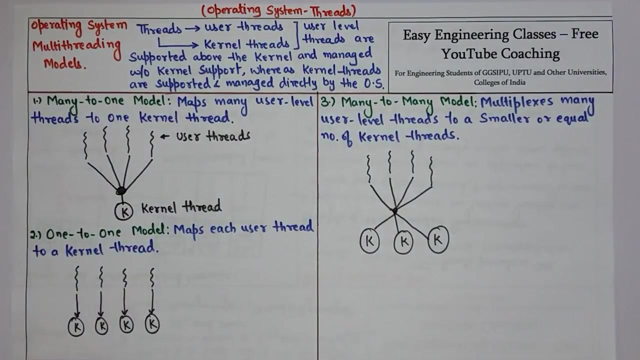 of operating system in which we have seen different kinds of multi threading models- many-to-one, one-to-one, many-to-many model- and also we have seen the benefits of multi threading and single and multi threaded process. so you can note the points from this video. thank you for watching the video please. you.